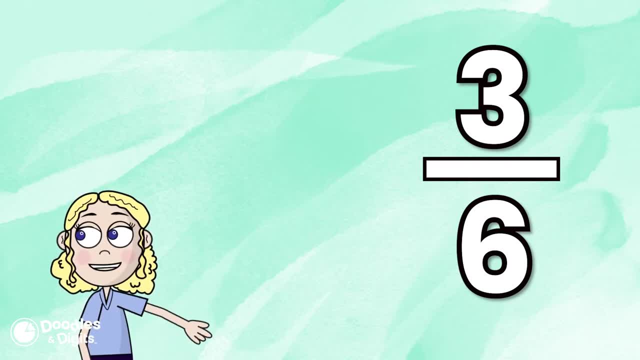 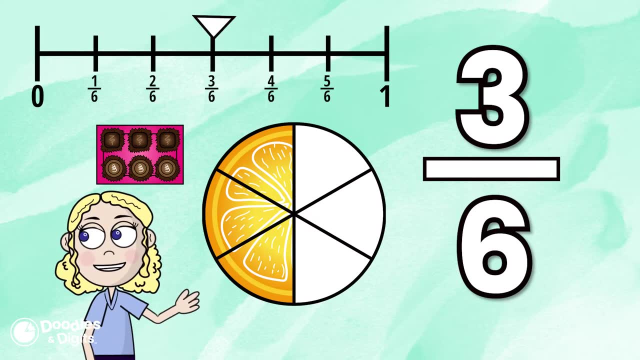 All right, so what is a numerator and denominator? Let's look at a fraction right here. Before we start, here's a couple different representations of this fraction. What do you notice? What do you think the numerator is and the denominator is? 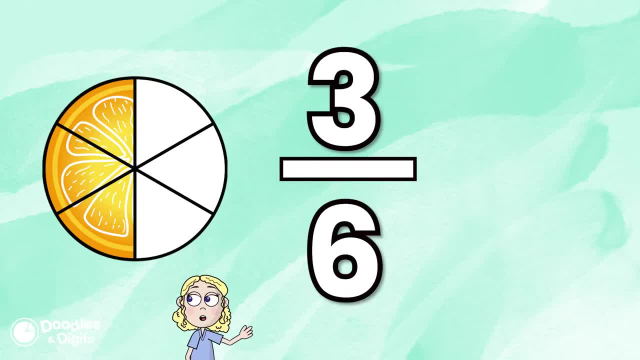 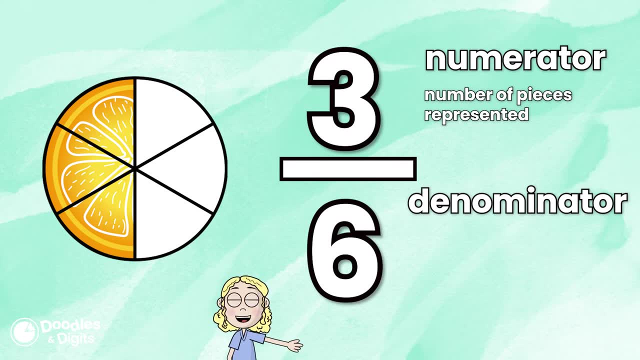 All right, let's look at a model that matches this fraction. The numerator is the number of pieces that is actually represented or that we have. The denominator actually represents how many equal pieces are in a whole- Something to remember when we're talking about fractions. 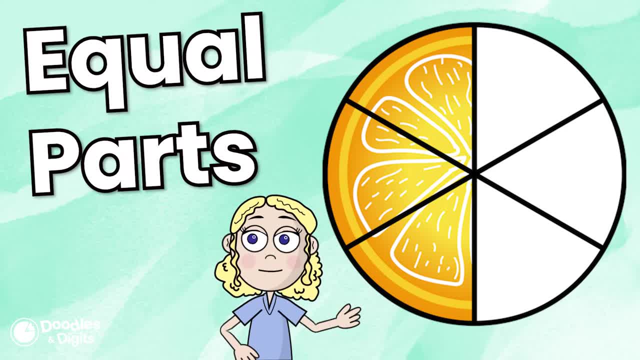 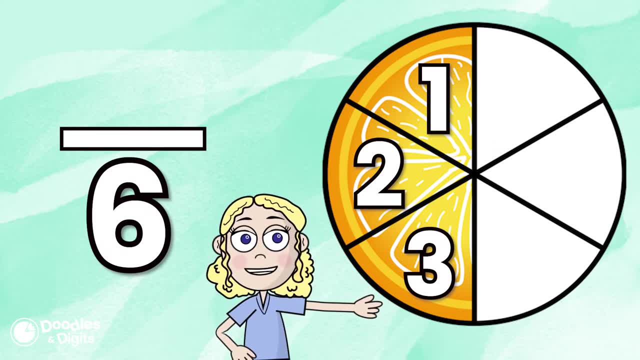 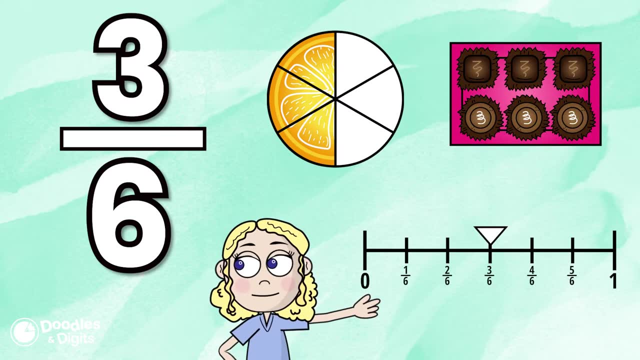 is, we are talking about equal parts, So the denominator is going to tell you how many equal parts we will have in the whole, and the numerator tells you how many equal parts you actually have. Here are multiple different representations of this fraction. Where do we see fractions in everyday life? Fractions are often used in measurements. 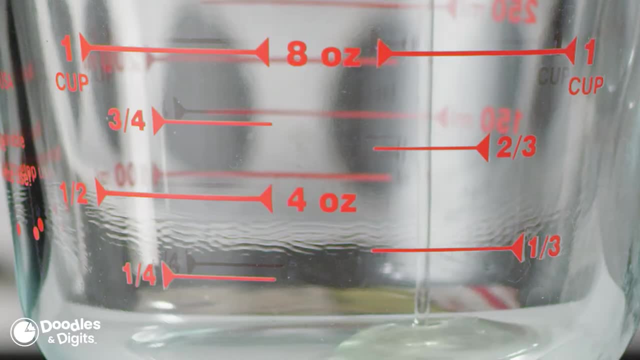 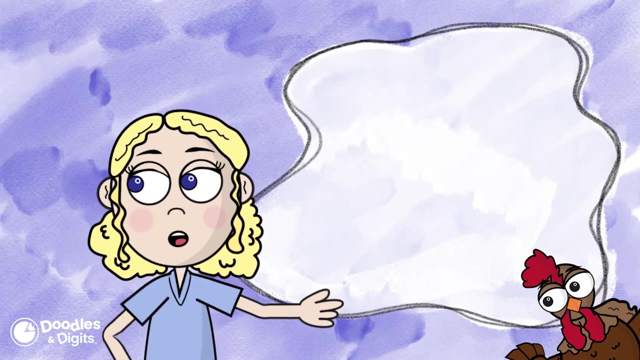 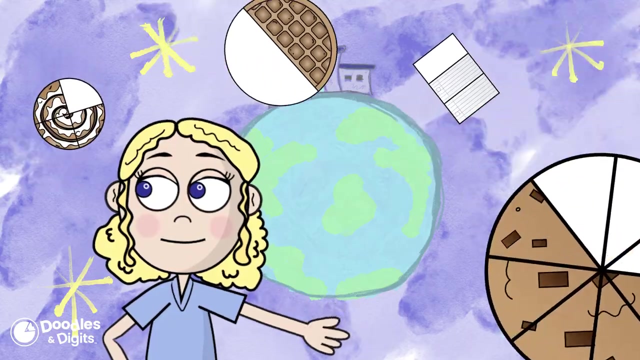 when baking, when adding, subtracting, Sometimes, when we're sharing, you'll think of fractions. For example, if we have a piece of pizza, we might be sharing the pizza. or maybe you're talking about a pie and there's 12 slices in a pie. Fractions are truly all around us. Fractions can. 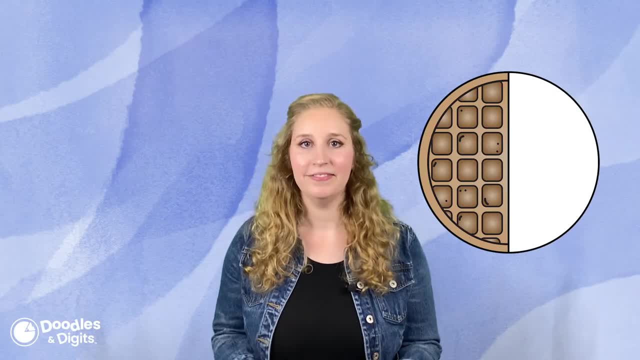 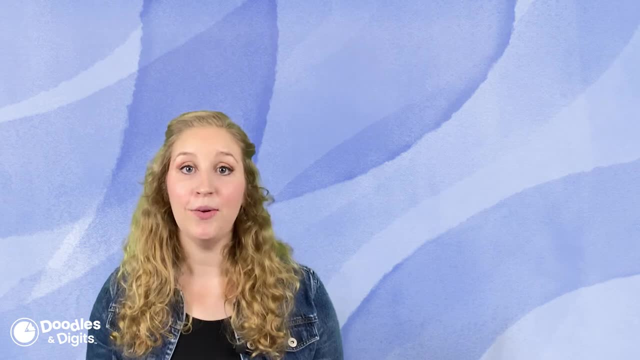 actually be displayed in a bunch of different ways. They can be in a model, they can be on a number line or they can actually be a part of a group. All right, I'm going to show you a couple different models and let's see if you can name the fraction. Let's try this one. This is a fraction. 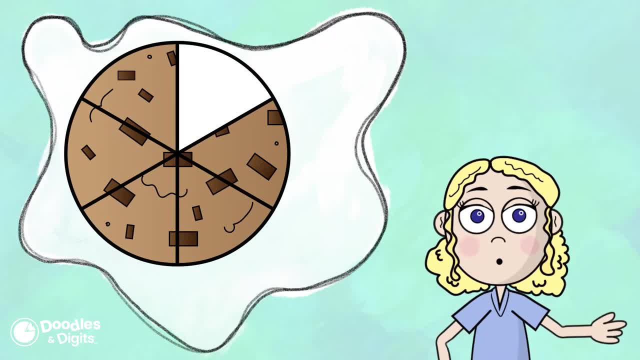 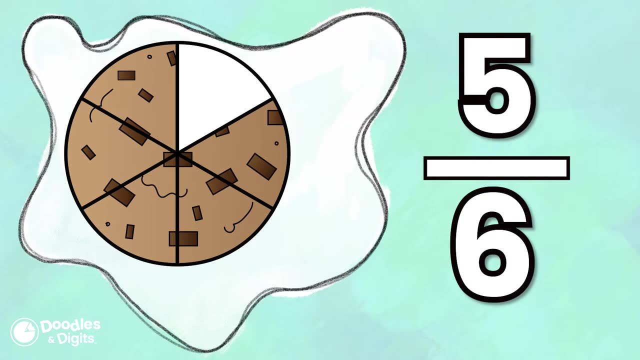 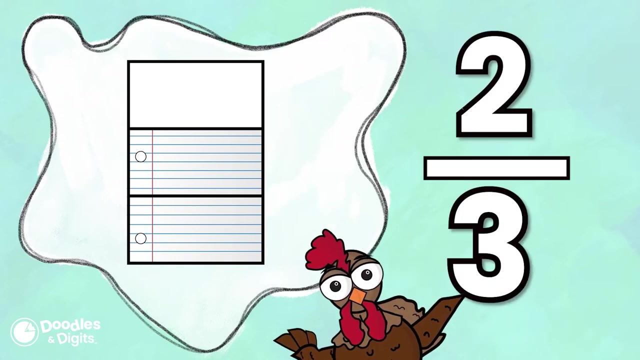 model. You might notice that this is cut into pieces. When do you think you would use these models when solving a problem? There are five pieces there and there's six pieces in a hole. So our fraction is five sixths. There's two pieces in the picture and there's three pieces in a hole. 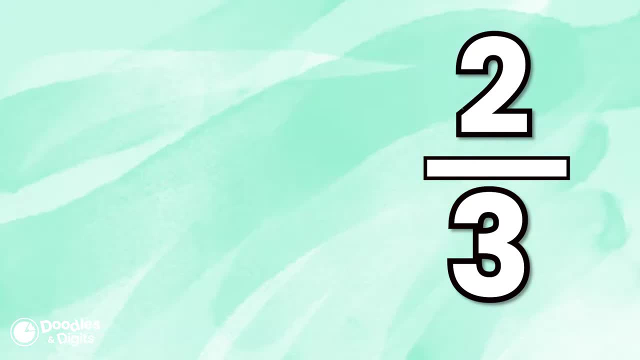 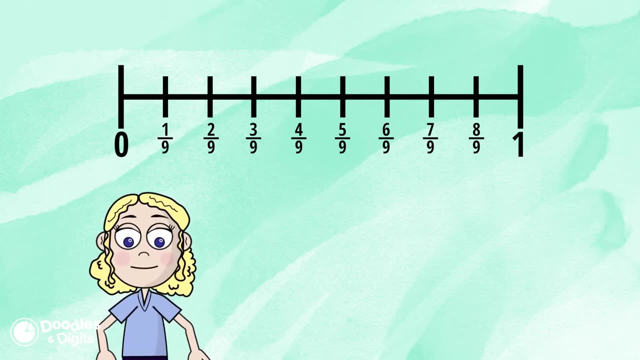 so our fraction is two thirds. You can also use a number line to show fractions. Let's look at a few number lines right now. Here is a fraction number line. What do you notice? What do you wonder? Between zero and one, it is cut into ninths. We're going to see how many. 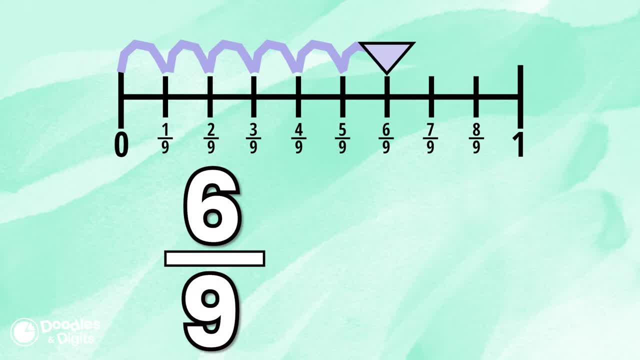 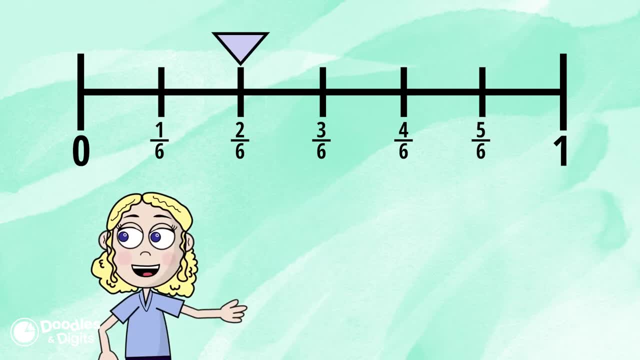 jumps we need to make to get to the arrow. We make six jumps, so our fraction is six ninths. Look at a few more fraction number lines. What's similar about all these fraction number lines? What's different? All right, let's look at this one. Between zero and one, it is cut into sixths. 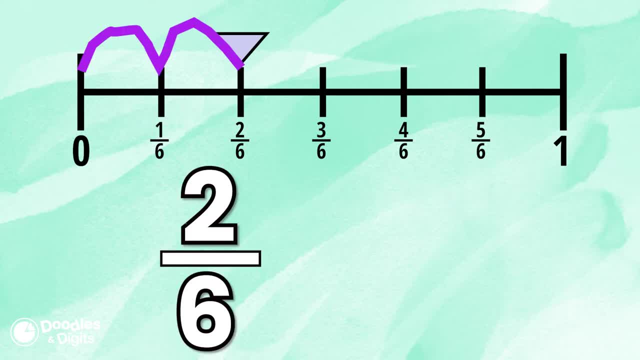 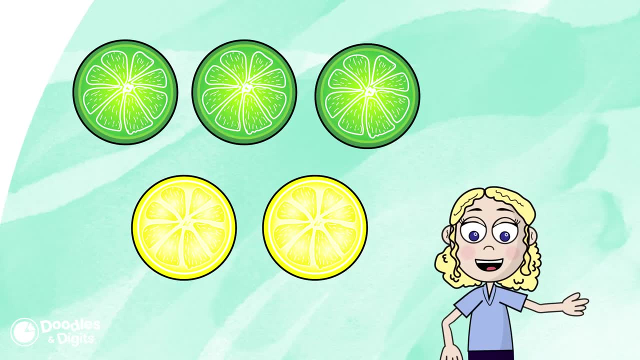 so now we're going to see where the arrow is. We're going to make two jumps and we'll get to two sixths. You can also show fractions. Let's look at a few other fractions. as a part of a group, Let's look at this picture right now. 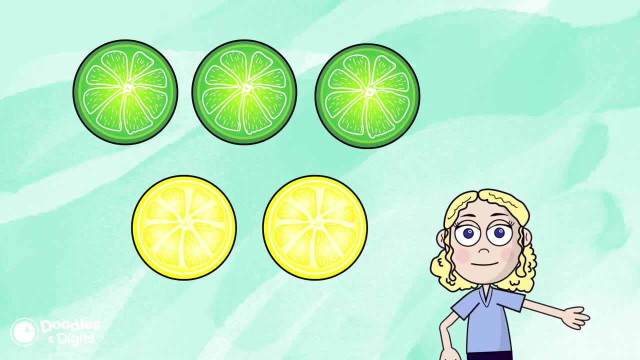 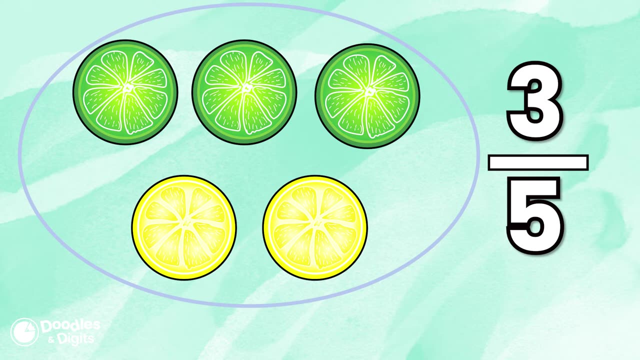 What fraction do you think this is showing? How do you think this represents a fraction? What do you notice? There's three lines. So in this group, three out of the entire group, which has five, are lines. You can also look at it the other way. you could say two. 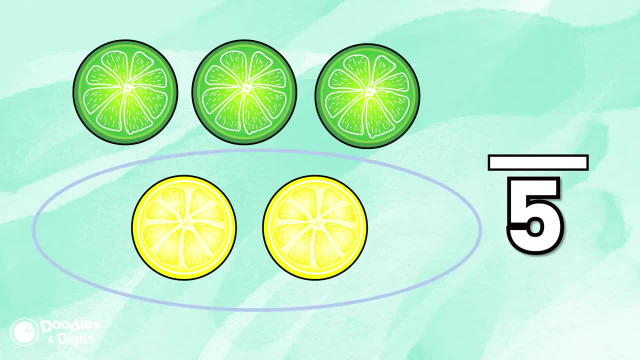 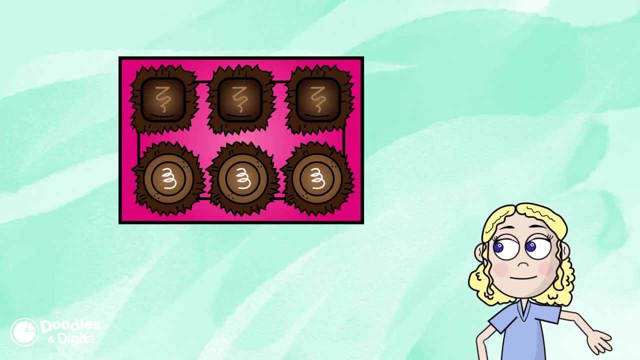 of the group is lemons— nar one. So 2 out of the 5. Five are lemons. Let's look at a few other parts of a group. What do you notice? What's the same, What's different? 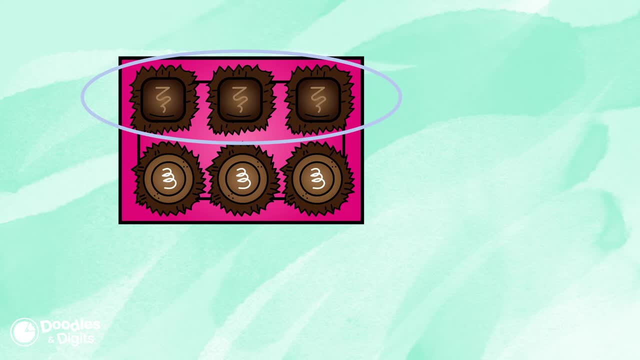 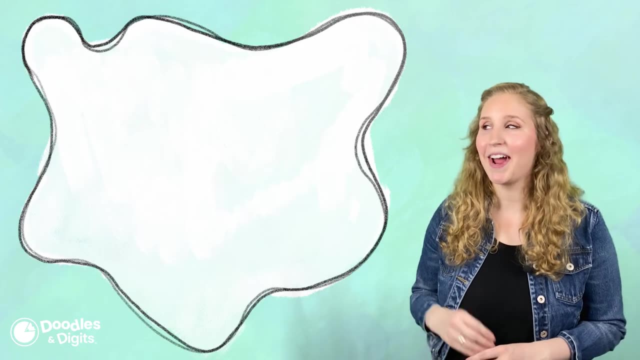 Three of these chocolates in this chocolate box are squares. There's six chocolates in the box total, so our fraction is 3- 6ths. All right, let's try this one. All right, so there's four chocolates total in this chocolate box. 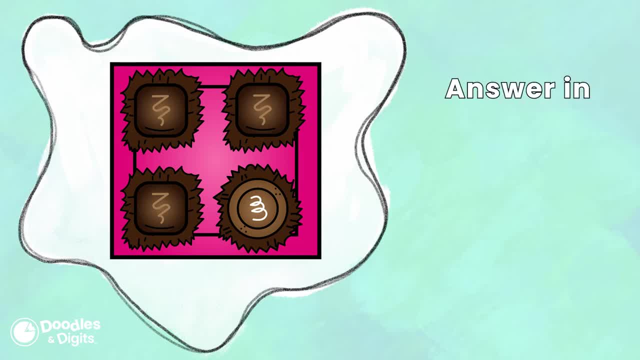 so our denominator is going to be four. Now we're going to say that there's three square chocolates, so our fraction's going to be 3- 4ths. If we were going to say the fraction of the circle chocolate, that would be 1- 4th. 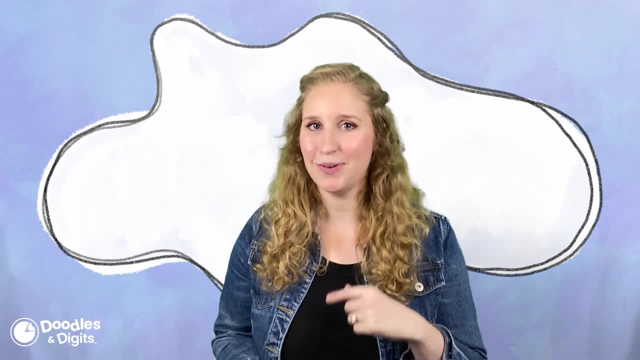 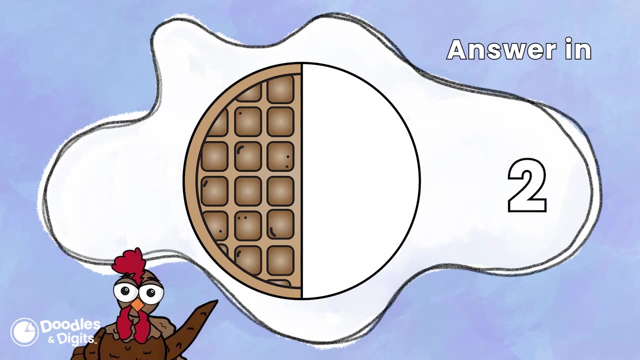 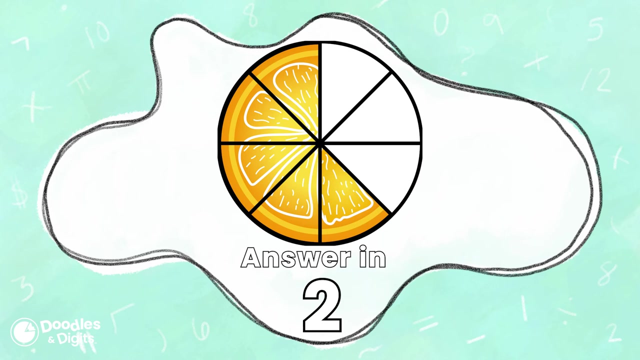 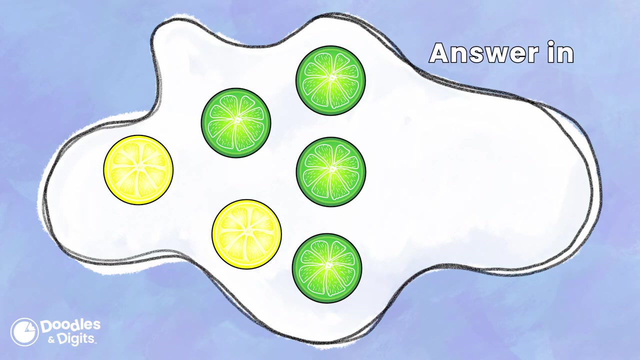 Now that we've named a couple fractions together, let's see if you can do a couple on your own. Number four would be two 1 4ths. Number five would be one 1 4th. One 8th. One 1 2nd.